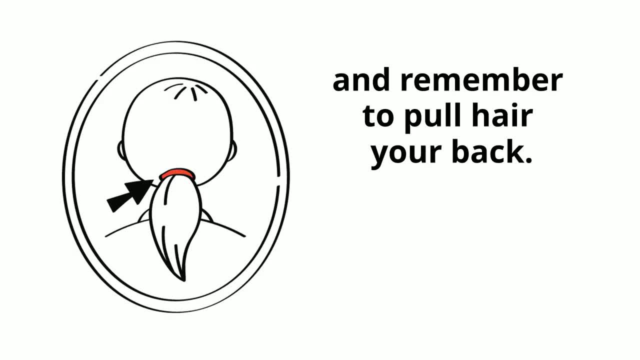 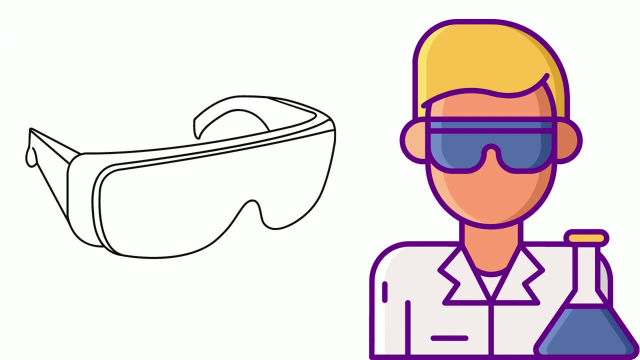 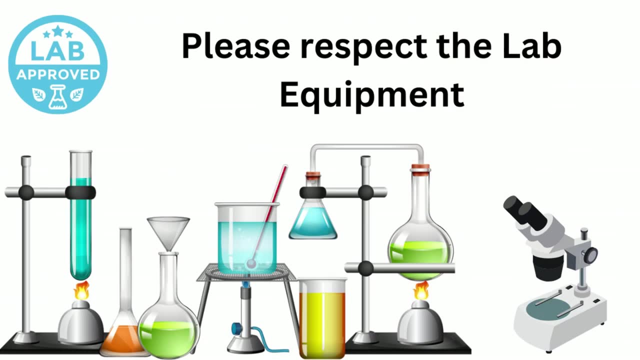 chemicals and other things do burn. Next, remember to wear your safety goggles. This just makes sense and, as my mom used to say, you don't want to poke your eye out. Next, be very careful with the laboratory Equipment and handle them as instructed. For example, the microscope carry with two hands. 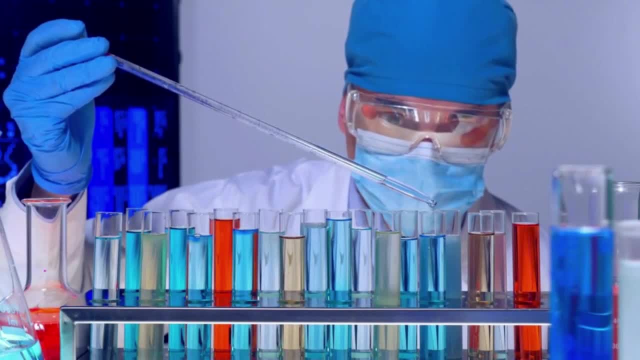 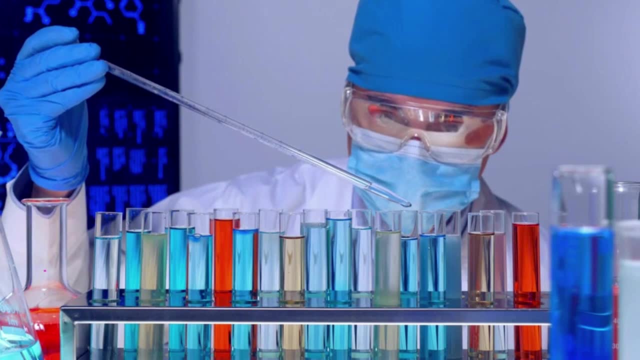 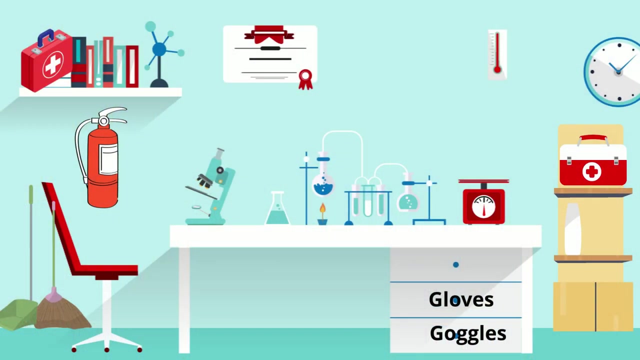 Next, be familiar with laboratory techniques involved for many of the activities before you attempt the activity. Some are a little complicated and you want to avoid spilling stuff or mixing the wrong chemicals. Next, it just makes common sense to locate and know where the safety. equipment is located. Next, be familiar with laboratory equipment and handle them as instructed. For example, the microscope carry with two hands. Next, be familiar with laboratory techniques involved for many of the activities before you attempt the activity. Some are a little complicated. 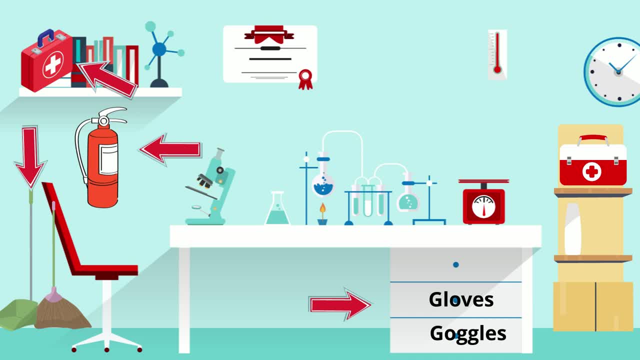 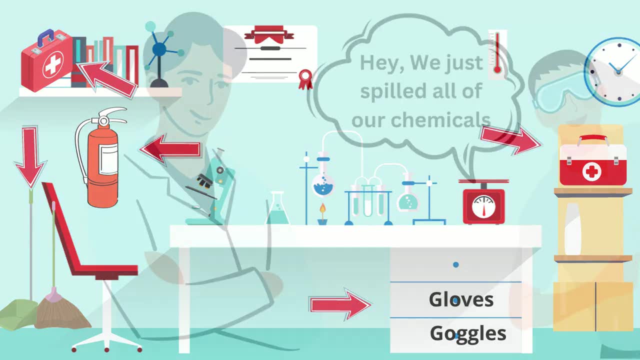 and you want to avoid spilling stuff or mixing the wrong chemicals. i've taught for many years and i have had cut hands and other things and it's nice to know where the first aid kit is. Next. what do you do? if you do have a accident? Report it immediately to the teacher. 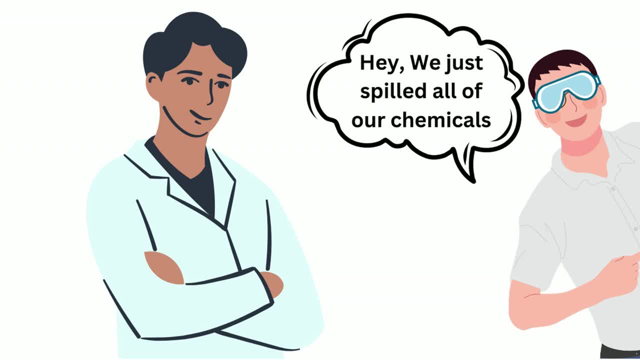 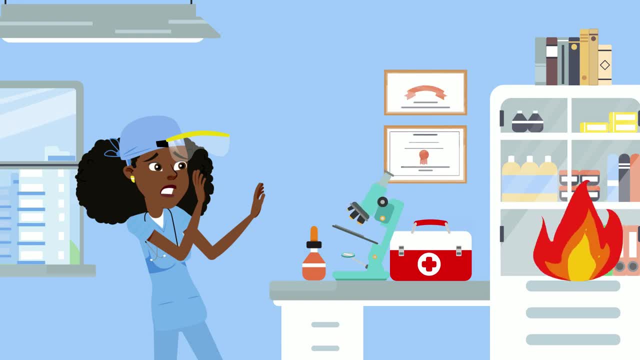 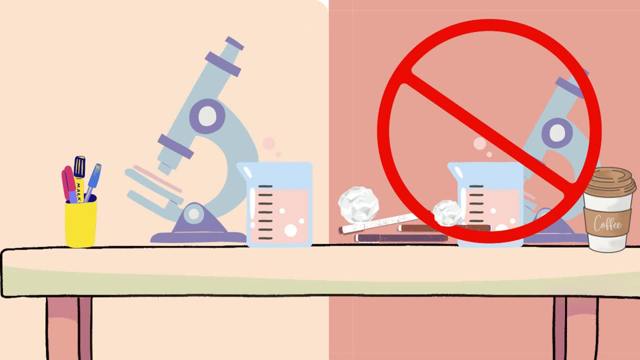 and also know where to go if help is needed. Next, be familiar with the procedure and what you need to do in case there's a fire in the laboratory. this one, your teacher will like you much more if you will work on keeping your workstation clean. 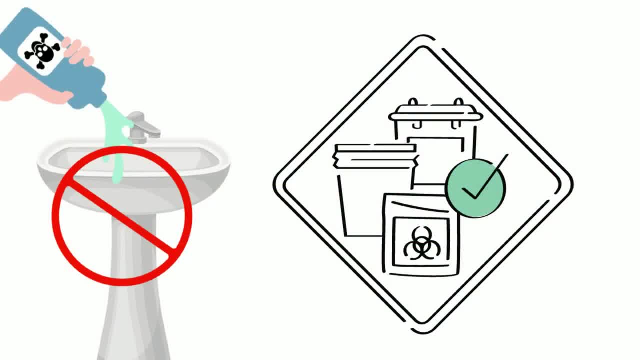 and organized. and finally, after you've completed your lab, you need to dispose of the chemicals. if you're using them properly, don't just pour them down the sink. your teacher will go over how you need to get rid of these materials and also return your materials and equipment to the proper places. 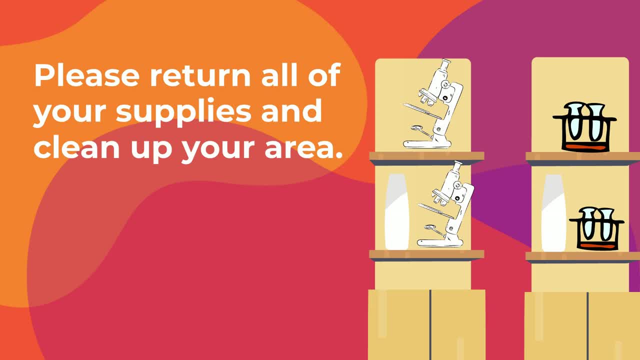 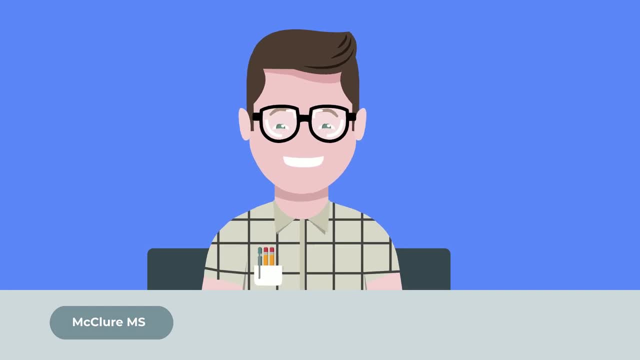 wherever your teacher has told you. i think if you can follow these simple common sense guidelines, everyone will be happy. thanks for watching and remember: kindness multiplies kindness. be kind to someone today.